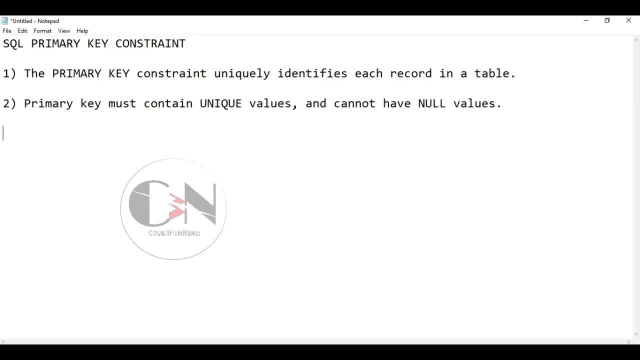 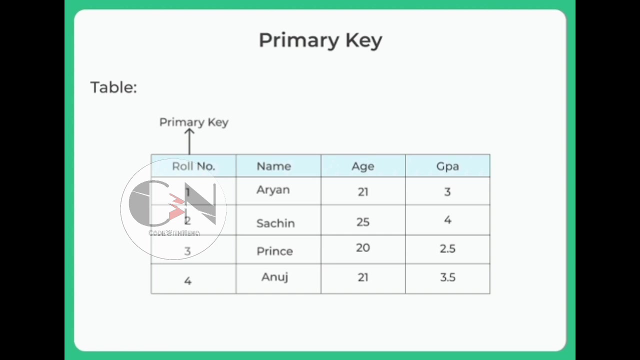 A table can have only one primary key and in the table this primary key can consist of single or multiple columns or fields. So let us check out an example of primary key. So this is a student table with role, number, name, age and GPA. 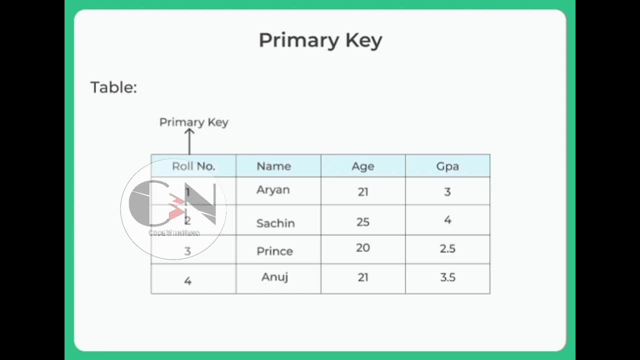 As we can see, there are different role numbers with different names of the student age and GPA. Here in this table the name, age and GPA can be repetitive, like Aryan and Anuj, both can be of the age 22.. Or Sachin and Prince can have same GPA of 4.. 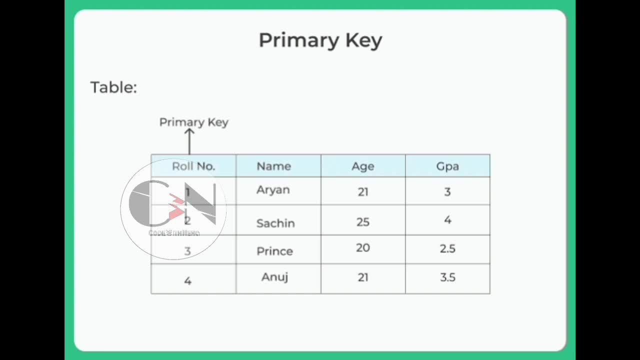 So which columns have the unique values? that will be the role number. So we can set the role number as our primary key. So for every students there will be one unique role number which will not be repetitive or duplicate. Let's check the syntax of the table. 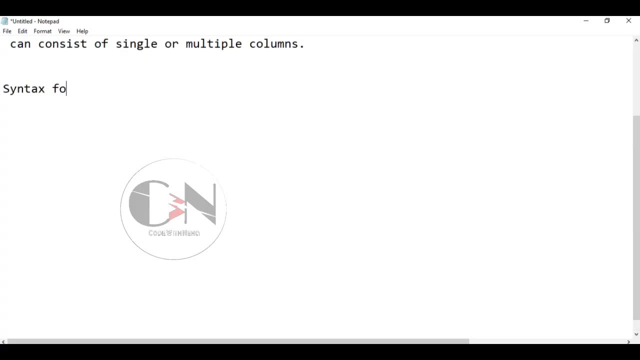 Let's check the syntax of the table. Let's check the syntax of primary key. So to set a primary key in a table, we can use the syntax in two ways. We use the create table syntax with the table name that we want. Then we define the column name with their data types. 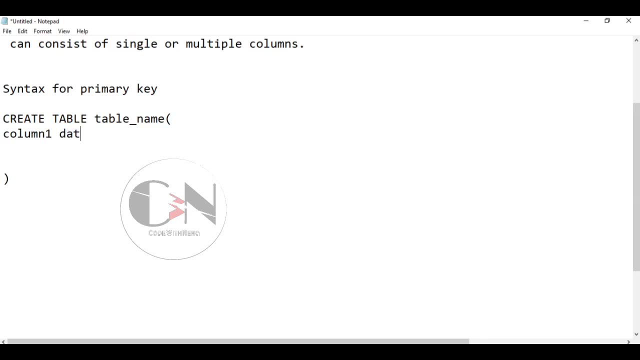 We can have as many column that we require. And, lastly, we define the primary key, that is, the column which we call table. And, finally, we define that we can have as many column that we want and every right will be repeated with example like this: 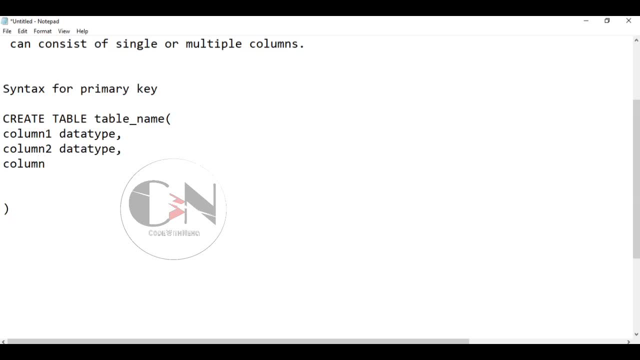 For example, could have one column that we call table and each column has 4 key is equal to all tables. So, as we can see, we have total of 36 cheques in our table. We can have a total of 36 cheques, which is equal to all tables. 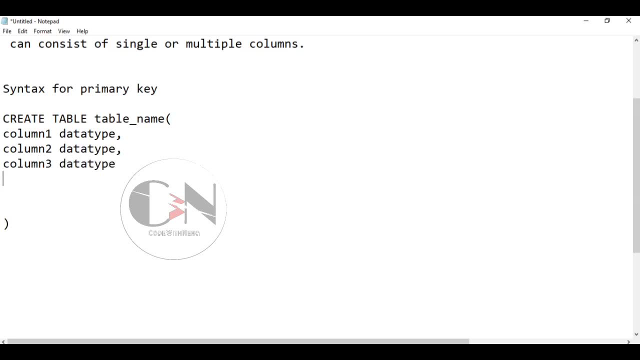 And that also can be automatically transferred in entry point pack at every table. This is the main text of size of our table, The first example of in a table that we have a table and in the example we have a table called as ilk. in this example ofuft by people in a table and in the example of 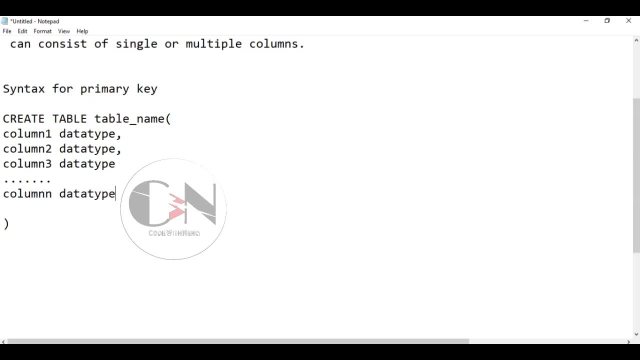 first example. we have a table which we call as primary key. So for this example, the table ofsize will be экside in every table and there will be at every pair of index is equal to heavens. then at the left, like and at: Thank you. 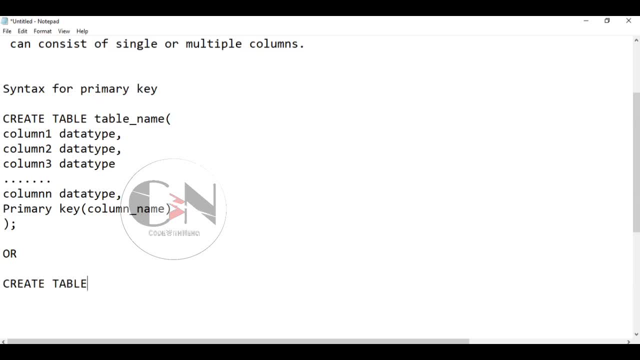 Or we use the create table syntax with the table name that we want. then we define the first column with data type as primary key, then followed by the remaining columns with their data type. Please note that this syntax is only for creating tables. 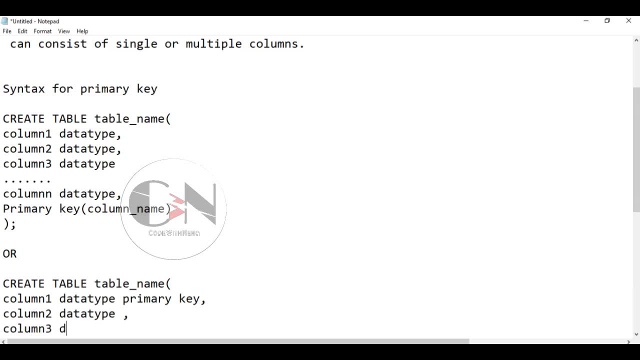 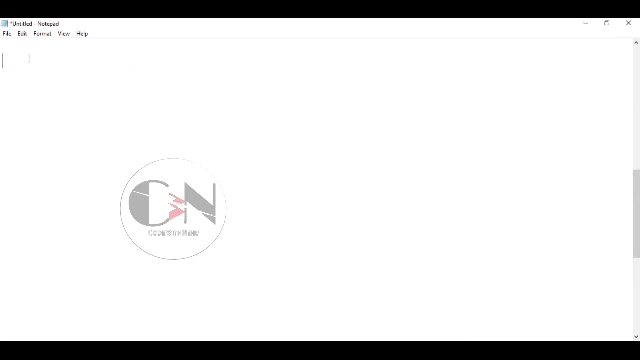 Before using create table: we use create database, then use database. Now, if you already have a table and you want to set a table, then you can use create table. If you already have a table and you want to set a column as primary key, you can use the alter command. 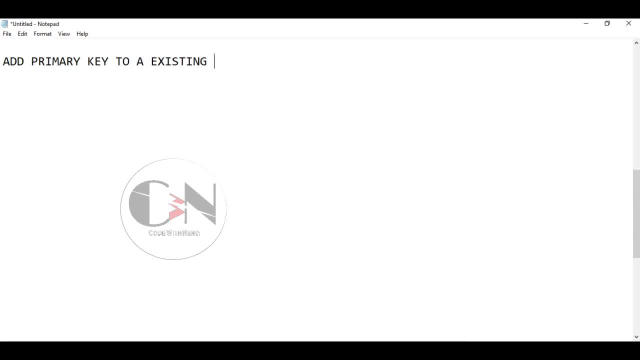 So for this we write the command as alter table. For this we write the command as alter table And the table name where you want to add the primary key And the syntax: add primary key with the column name. And the syntax: add primary key with the column name. 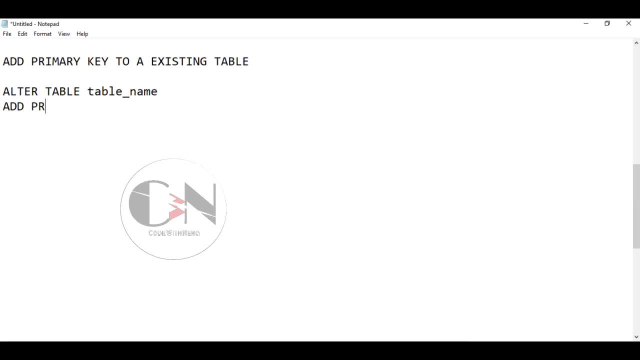 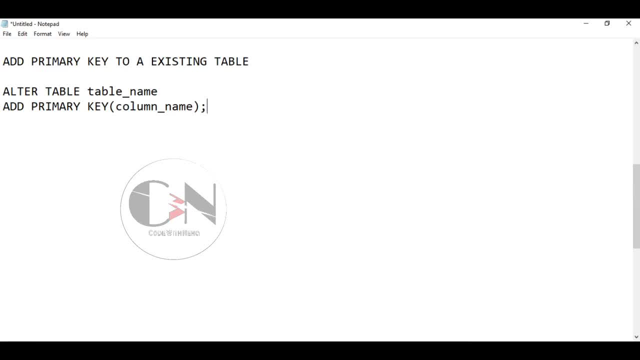 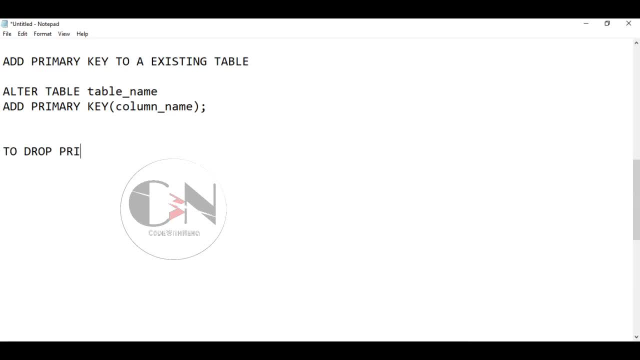 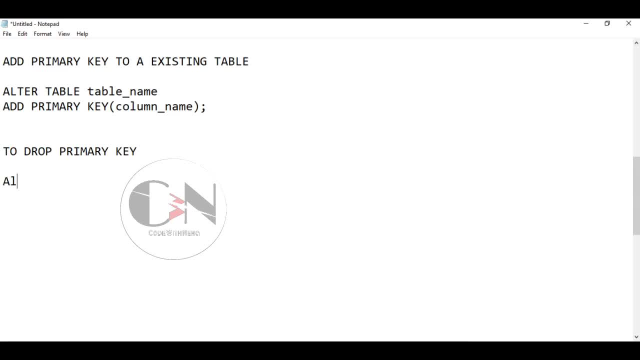 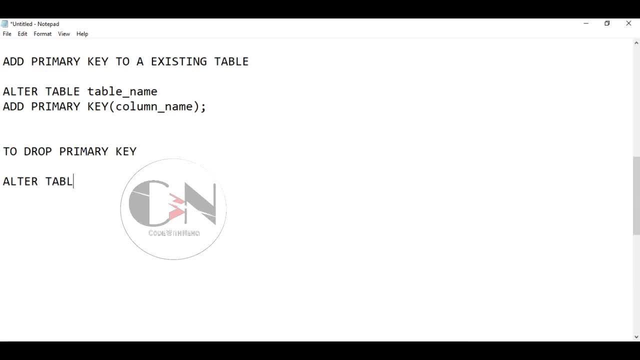 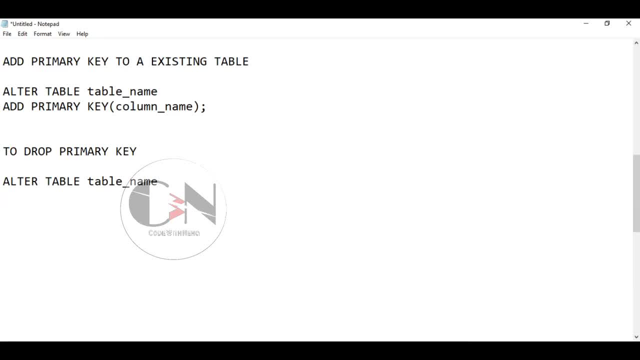 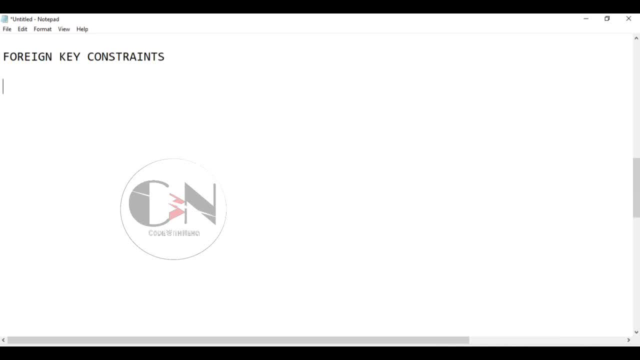 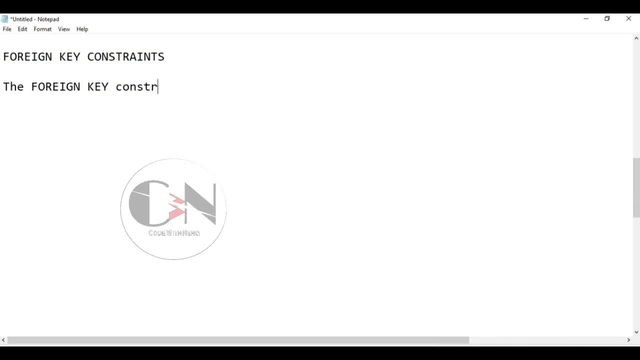